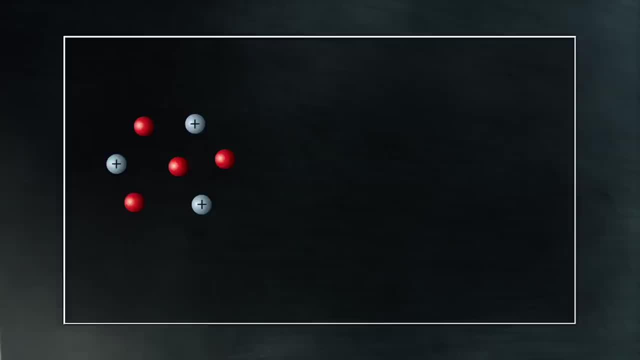 of nuclear energy. During fission and fusion, a small amount of mass is converted into binding energy, some of which is released as radiation that we can use as a source of heat. Let me start by going back to the example of that helium atom, The nucleus of most helium. 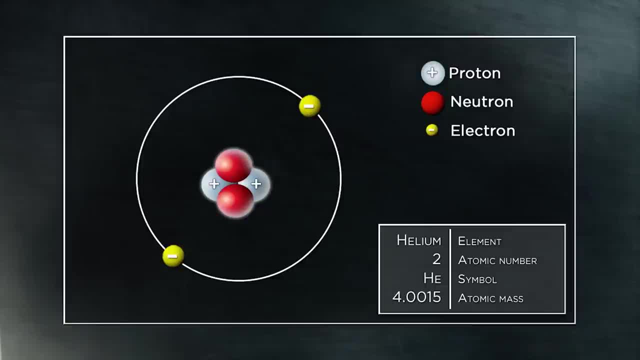 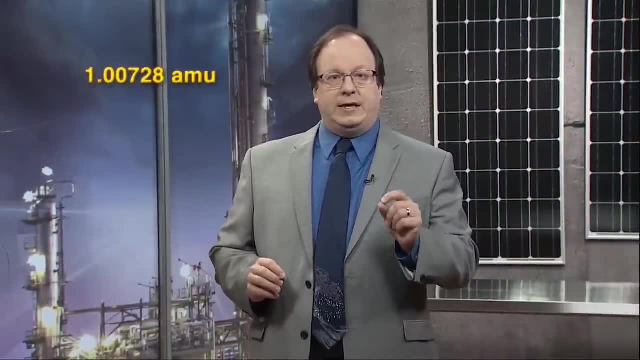 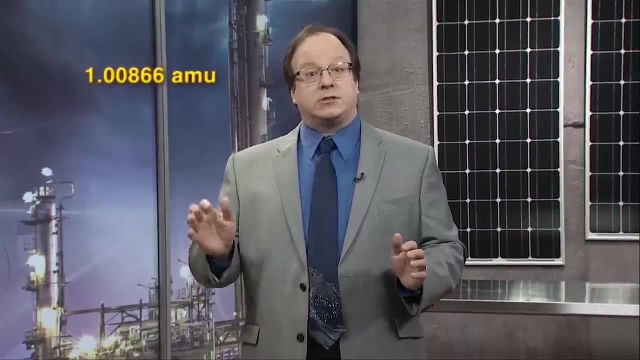 atoms contains, as I said, two protons and two neutrons, And we know the masses of individual protons and neutrons. A proton is 1.00728 atomic mass units. A neutron is 1.00728 atomic mass units, slightly larger. So if you added 2 protons and 2 neutrons together, you would get 4.0319 atomic mass units. Sorry for all of the decimal places, but I need to include them to make a point here. Okay, 2 protons, 7 patrons, 4.0319 atomic mass units. However, if you look at the nucleus, 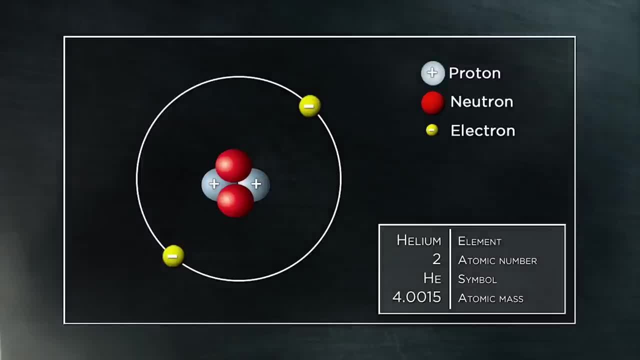 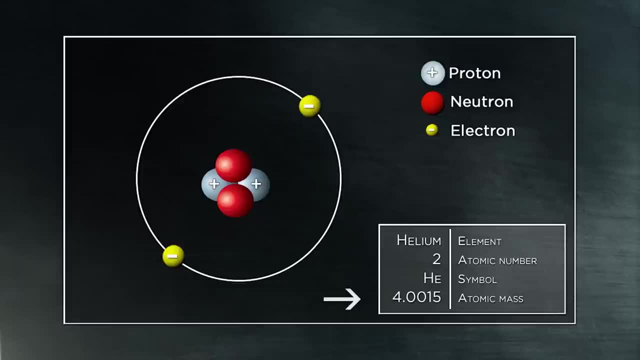 of a helium atom, 7 artifacts, 7 days of impl mindful hours. But if you 비용 telesano, not what you get. Sure enough, you have two protons and you have two neutrons, but the mass is less. It's now 4.0015 atomic mass units. This is less than the mass of the separate protons and 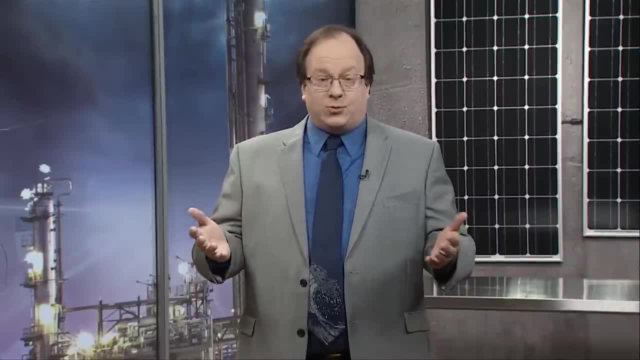 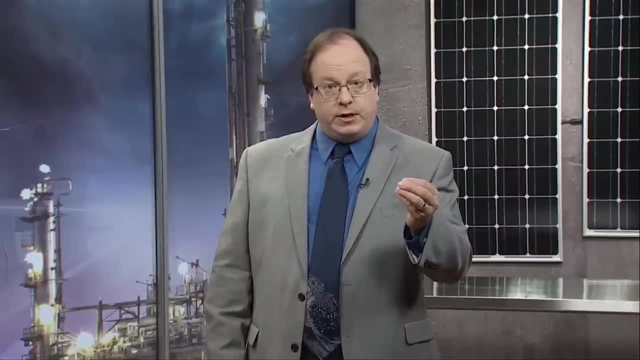 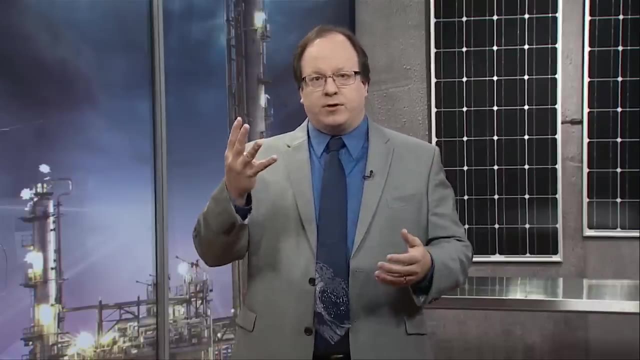 neutrons, And this is very strange. This is one case where the whole is actually less than the sum of the parts. The difference between the two 0.0304 atomic mass units, This is a little less than 1%. So this is strange. You take four particles, you put them together and you 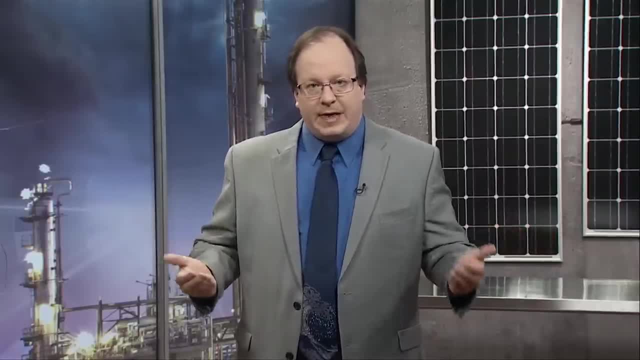 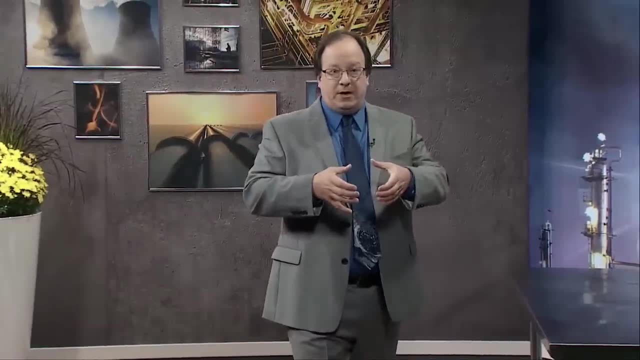 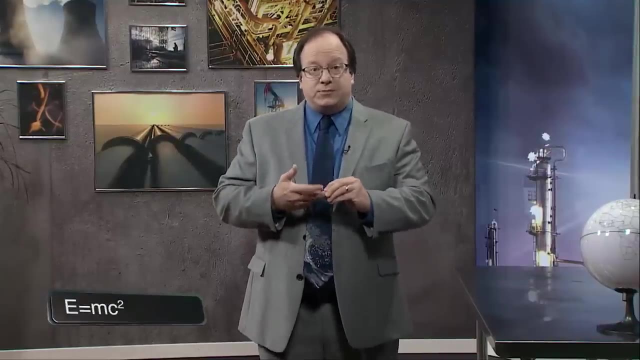 suddenly lose 1% of their mass. Where did that missing mass go? Well, it went into the energy needed to bind the particles together, And you can calculate exactly how much energy that is. After all, energy is conserved, And we know that Einstein's equation E equals mc squared will. 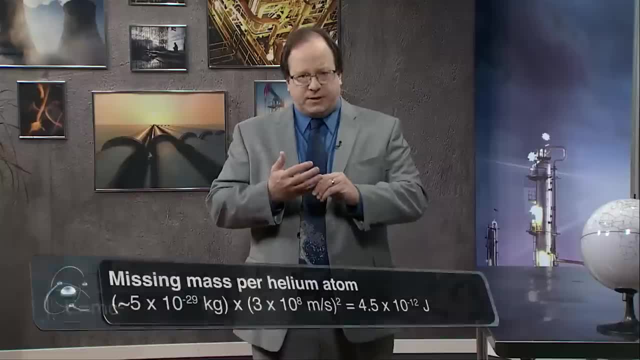 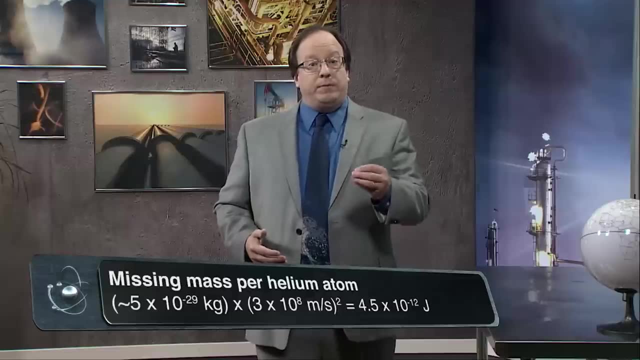 tell us how much energy we get from the mass, The missing mass turns out to be about five times 10 to the minus 29th kilograms. That's incredibly small, But when we multiply it times the speed of light squared, which is three times 10 to the eighth meters per second squared, that's a very 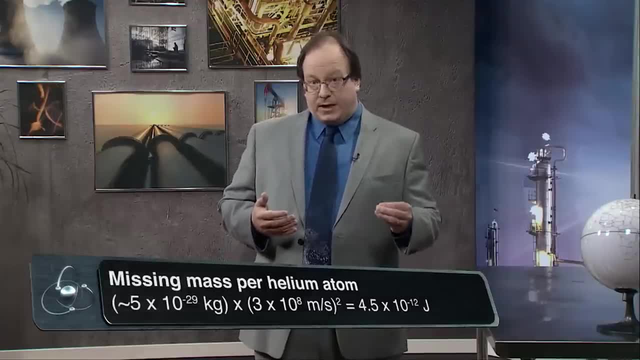 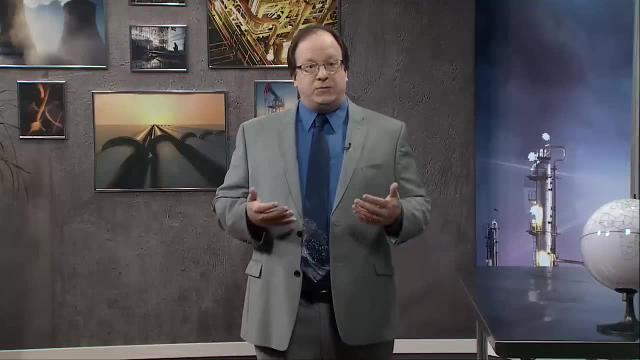 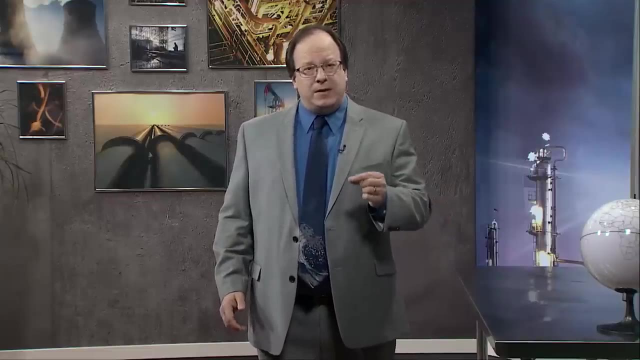 big number. we now get four and a half times 10 to the minus 12 joules That's for each helium atom. So joining the neutrons and the protons to make the helium nucleus converts the mass into energy, a lot of energy. One gram of helium made from fusion. 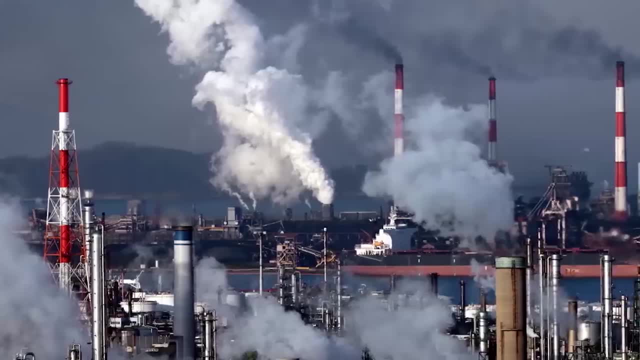 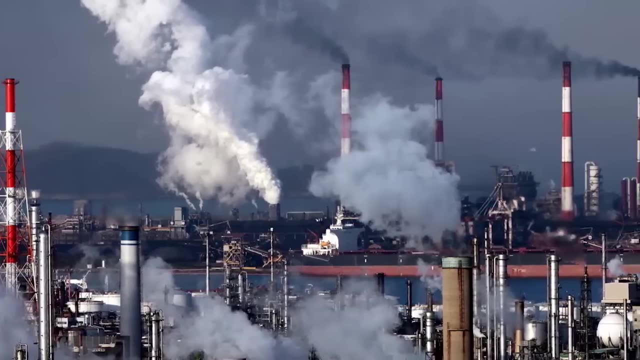 that's about the weight of an almond- generates the same amount of energy as you get from burning 23 million grams of coal- 23 tons of coal from something the size of an almond. A nuclear power plant is similar to a coal-fired plant. 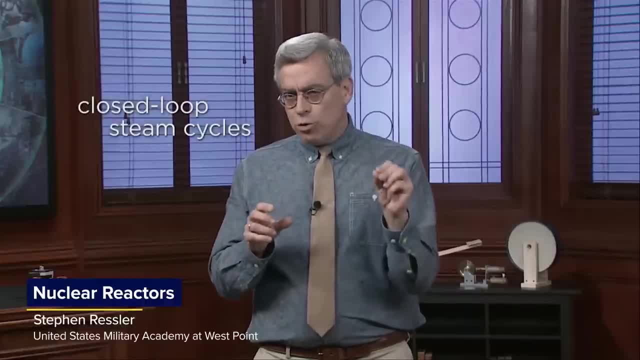 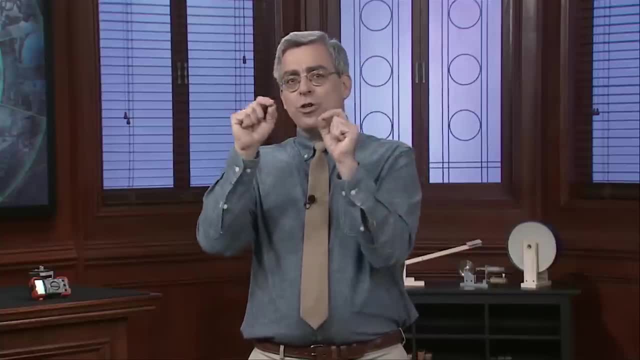 in the sense that both use closed-loop steam cycles to spin turbines. The big difference is simply that the source of energy used to produce the steam is different. It's chemical energy for a coal-fired plant. It's energy for a coal-fired plant. It's energy for a coal-fired. 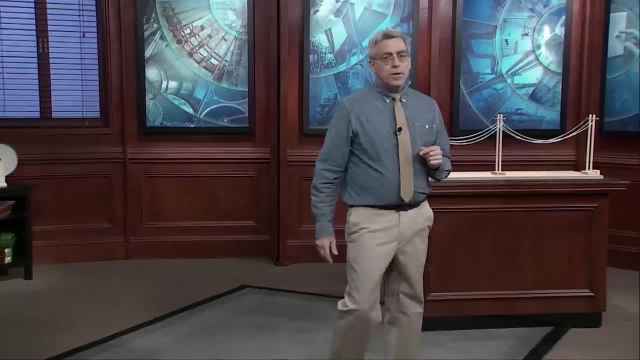 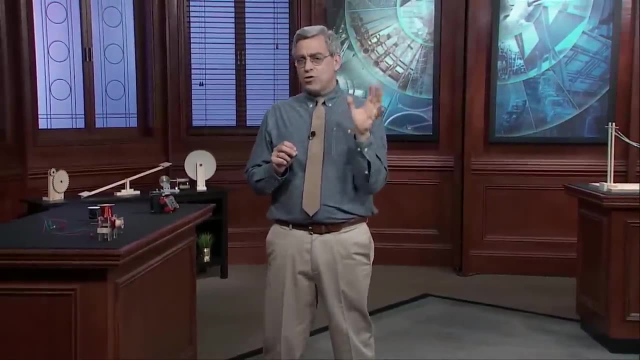 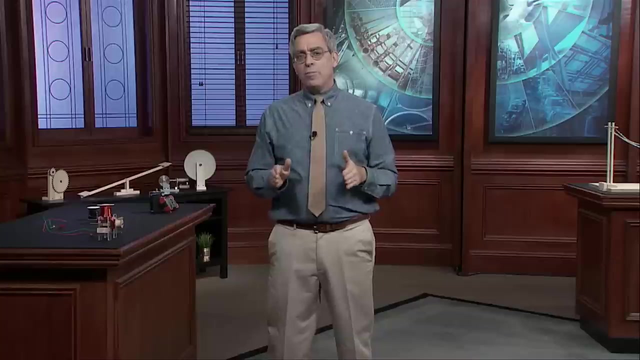 plant Nuclear fission. for a nuclear plant, Nuclear fission, the splitting of atomic nuclei depends on the unique behavior of certain heavy elements called fissile materials, which are used as nuclear fuel. By the way, the word fissile means easily split, and so 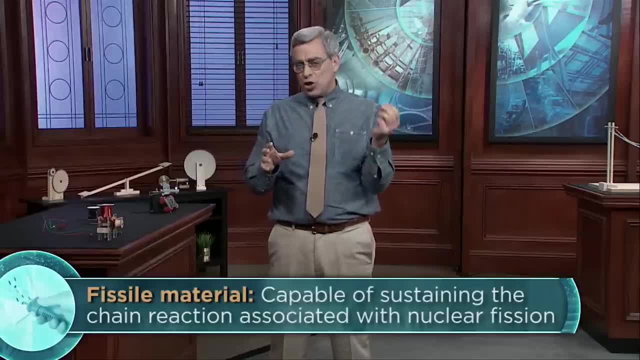 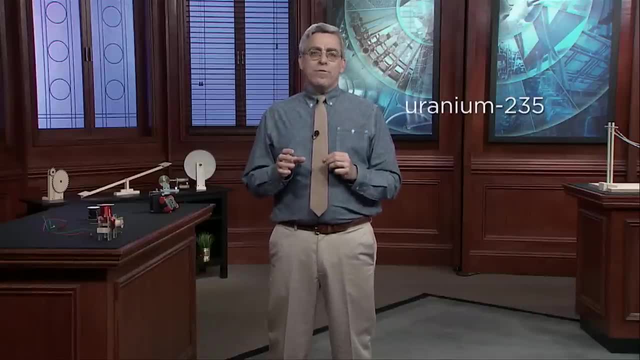 a fissile material is one that's capable of sustaining the chain reaction associated with nuclear fission. The most common fissile material is uranium-2,000.. The most common fissile material is uranium-2,000.. When the nucleus of a U-235 atom is struck, 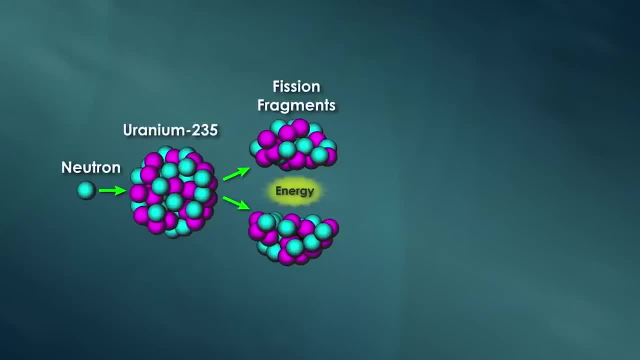 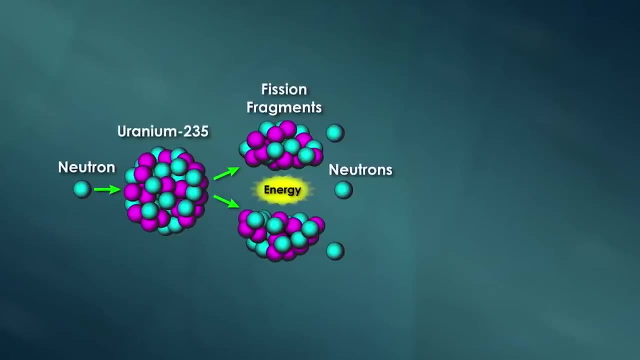 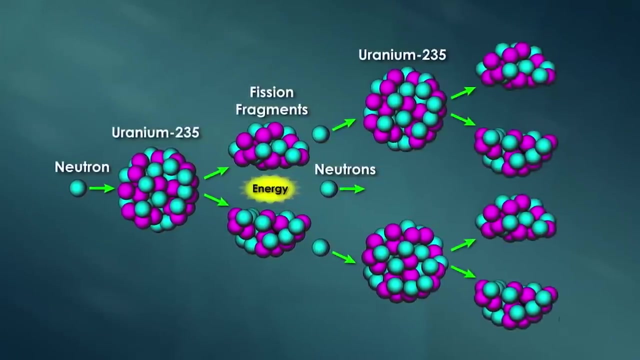 by a neutron. it breaks apart, releases energy and emits a few free neutrons. If a sufficient quantity of this material is assembled in one place, the neutrons emitted by the fission of one nucleus will encounter adjacent nuclei, causing them to split, release energy and. 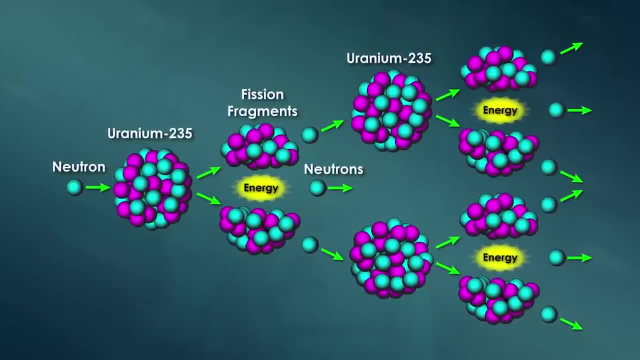 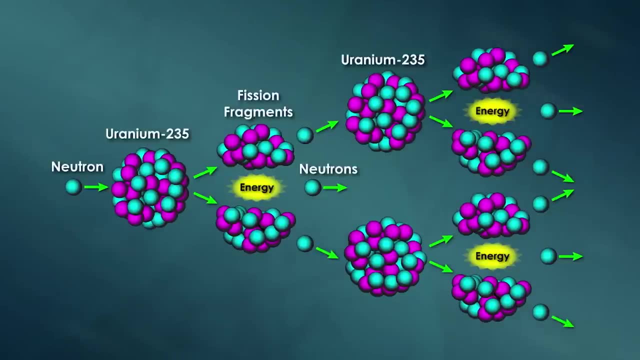 emit more neutrons. As this process continues, progressively more free neutrons cause the fission of progressively more nuclei, And the result is a nuclear chain reaction – self-sustaining fission. If this chain reaction is controlled, we have a very potent source of energy. If it's uncontrolled, we have a nuclear explosion. But how does this reaction get started in the first place? Well, uranium-235 experiences a small amount of spontaneous fission – a natural form of radioactive decay that releases a few neutrons. 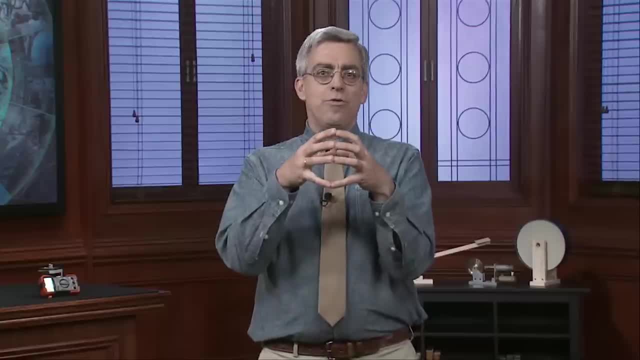 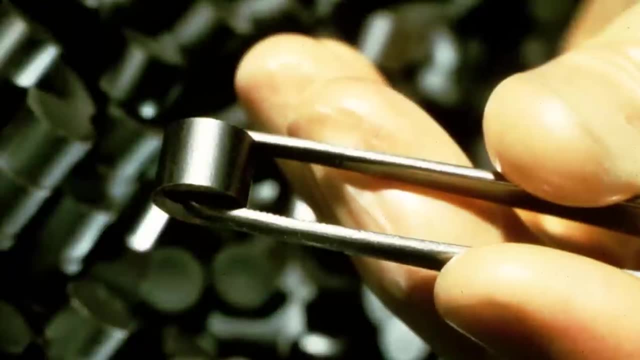 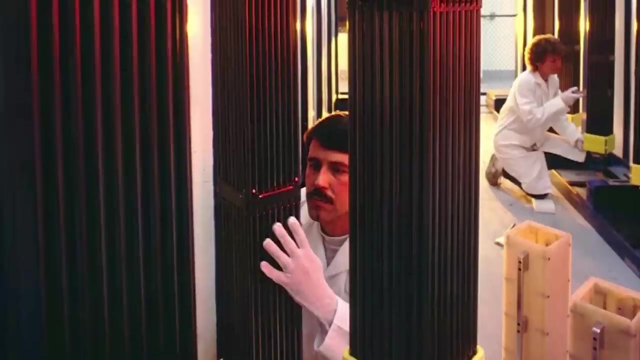 So we really only need to assemble a critical mass of uranium-235, and this natural emission of neutrons will set the nuclear chain reaction in motion. Nuclear fuel is prepared for use in a reactor by molding uranium into small pellets, which are then sealed inside metal tubes to create fuel rods. 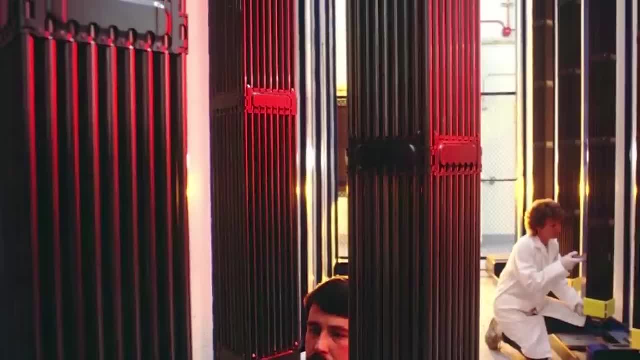 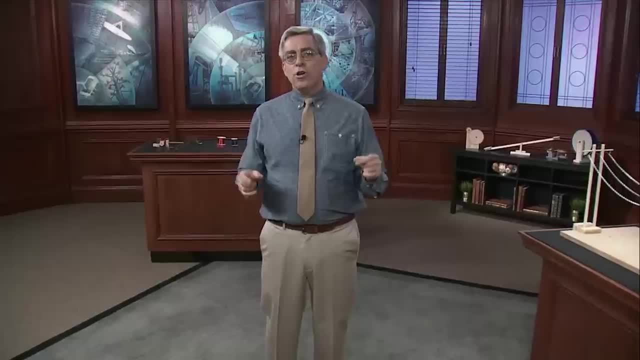 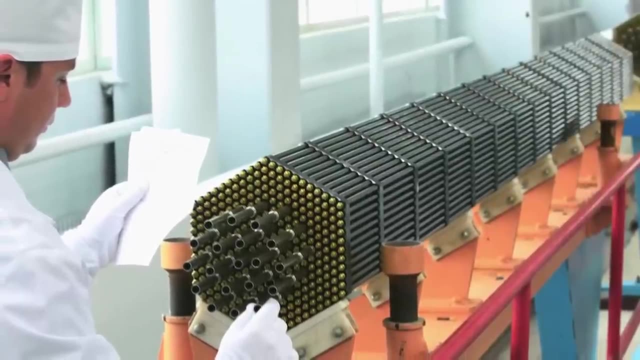 The tubes are made of zirconium alloy, used because of its corrosion resistance and low neutron absorption. The purpose of the tube is to contain the uranium pellets, so fragments can't break away and contaminate the reactor coolant. The fuel rods are assembled into bundles of about 200 each, like this: 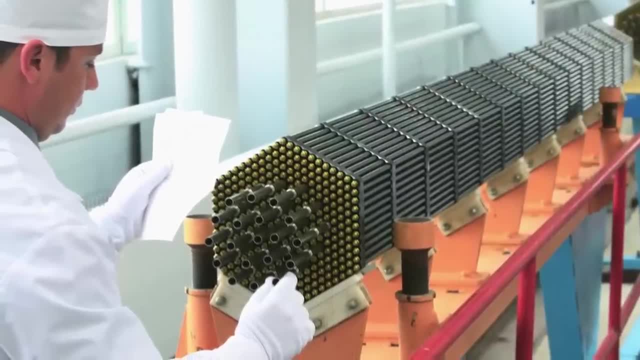 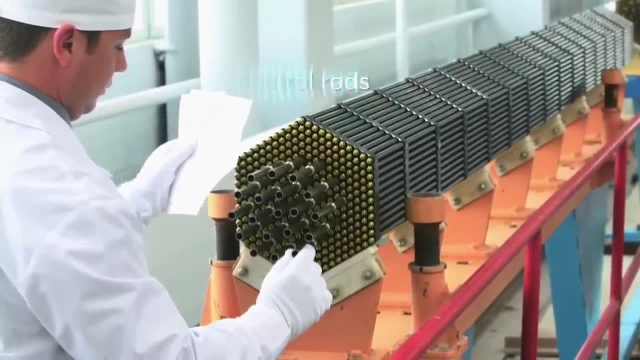 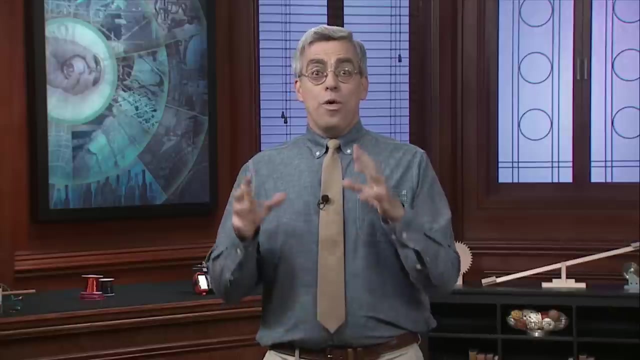 And about 150 such bundles are then combined to form the reactor core. These holes in each bundle allow for the insertion of control rods – cylindrical bars made of boron carbide, a material that's particularly effective at absorbing neutrons. When the core is completely destroyed, the reactor is destroyed. When the control rods are inserted into a fuel bundle, they absorb enough free neutrons to prevent the fission reaction from sustaining itself. Thus they keep the nuclear reaction from getting out of control. When they're withdrawn, they allow the reaction to proceed. 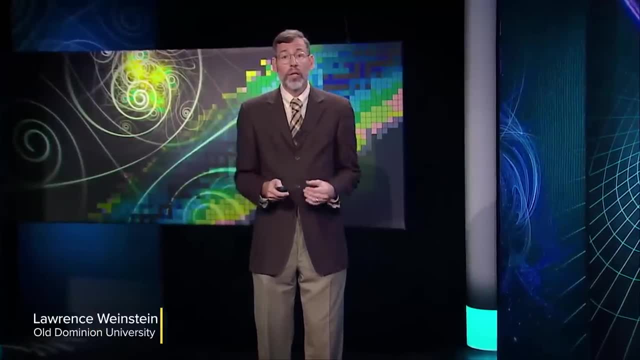 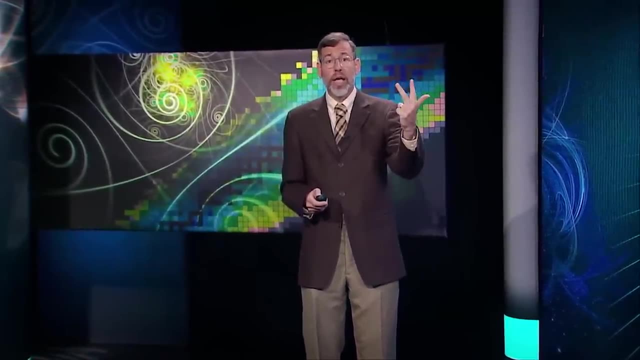 How do we turn heat into electricity? Well, we have to obey the three laws of thermodynamics. The three laws of thermodynamics are: you can't win, you can't break even and you can't quit. Or what it really means is: you can't win and it's a failure. 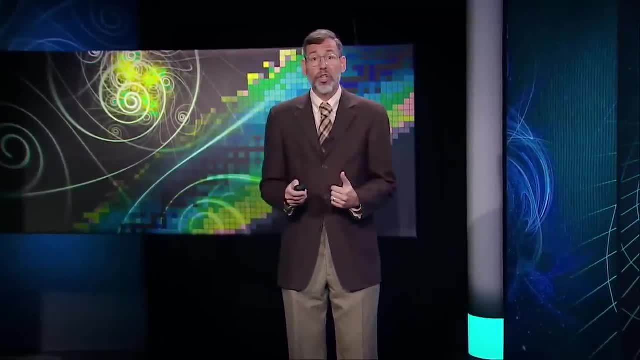 And the three laws of thermodynamics are: you can't win, you can't break even and you can't quit. The first one is: you can't win. energy is conserved. You can't break even, which says that entropy increases or the amount of useful energy decreases. 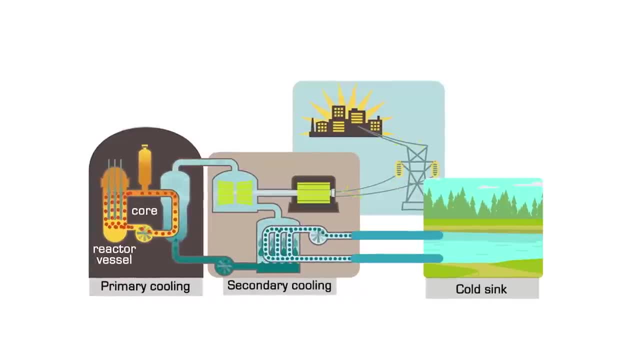 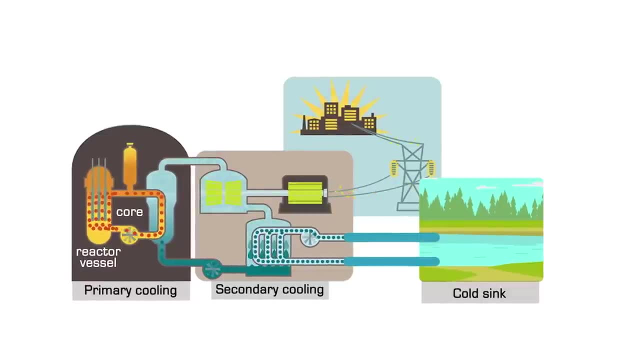 and you can't quit. So what do we do? We use the heat to boil water, to turn a turbine, to spin a generator, And we need a cold sink to dump the waste heat into. That cold sink can be a river, a lake or an ocean. 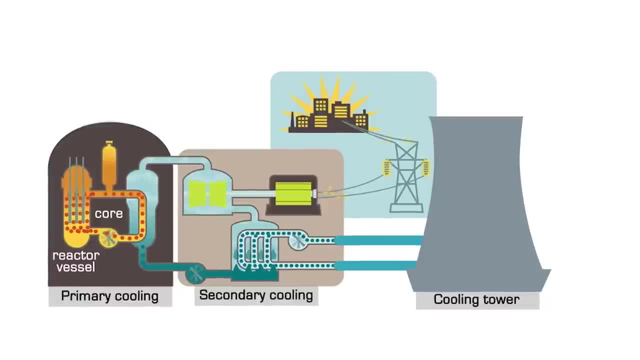 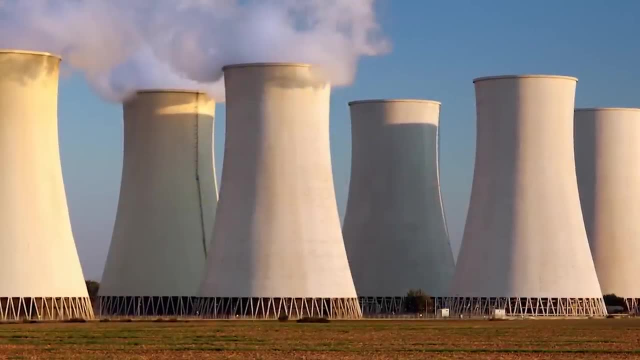 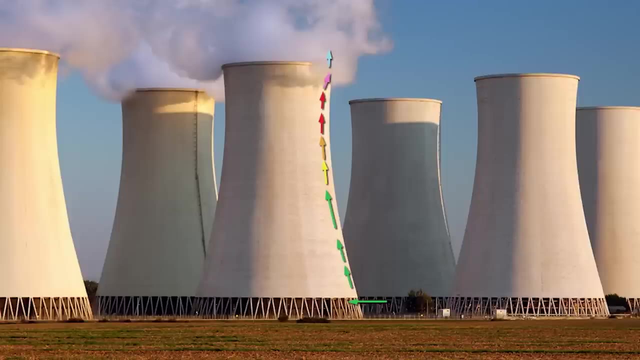 Or we can use a cooling tower. Cooling towers get rid of some of that waste heat by evaporating a lot of water, And that peculiar shape of cooling towers that you see on the skyline is there to maximize the airflow, And the thermodynamic efficiency is about one-third, and so that means that two-thirds. 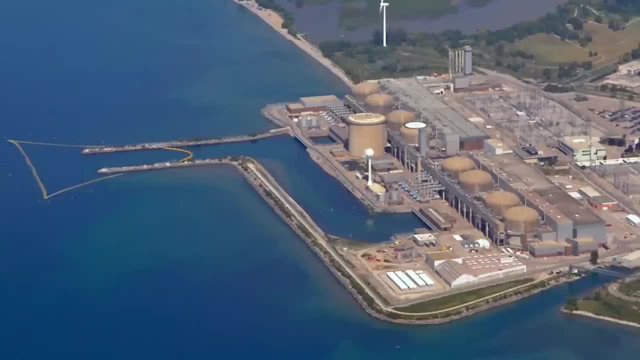 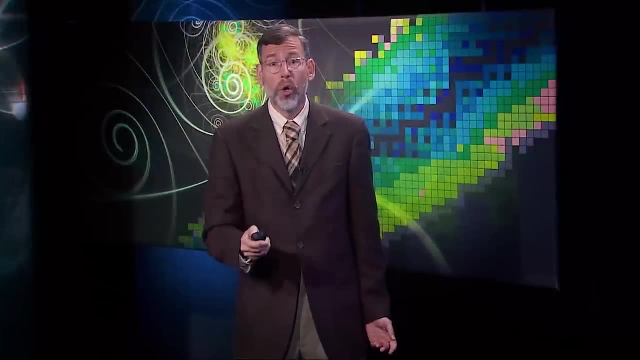 of the energy has to be dumped into rivers, lakes or oceans or up the cooling tower, And that's due to the limitations of thermodynamics. We use the same process for coal. We use the same process for coal, natural gas and nuclear power to turn heat into electricity. 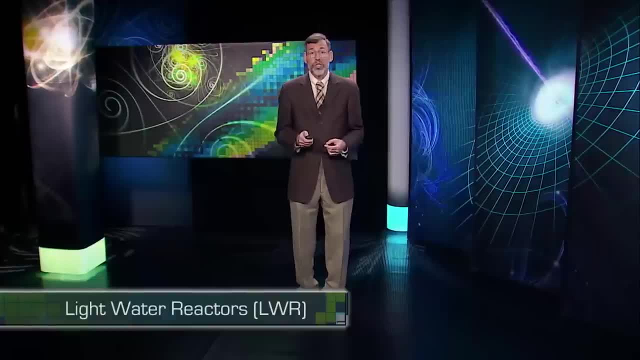 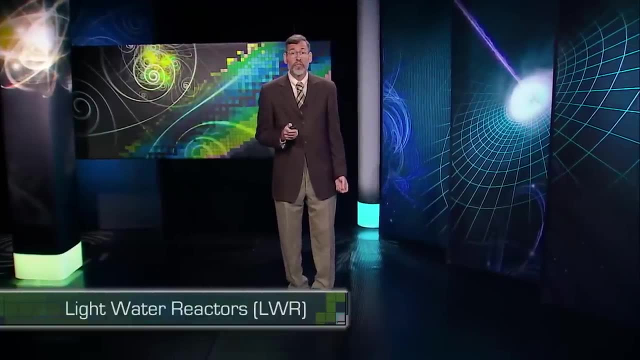 What kind of reactors do we use today? We use light water reactors, so that's regular hydrogen, not deuterium. The water is both the moderator and the coolant, And these were originally developed for the US Navy under the guidance of Hyman Rickover. 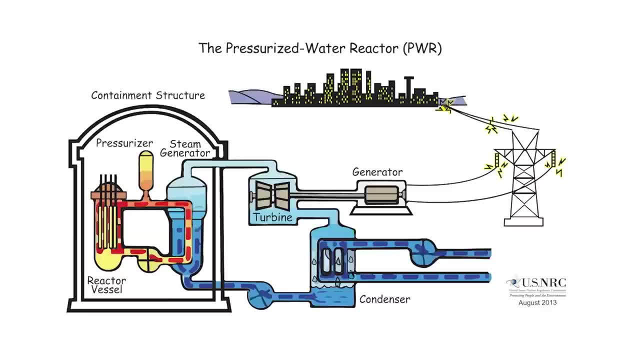 There are two general types of light water reactors. There's the pressurized water reactor, where the water is under high pressure so it doesn't boil. Higher pressure means a higher boil, And so the primary cooling water then has to transfer its heat to a secondary water. 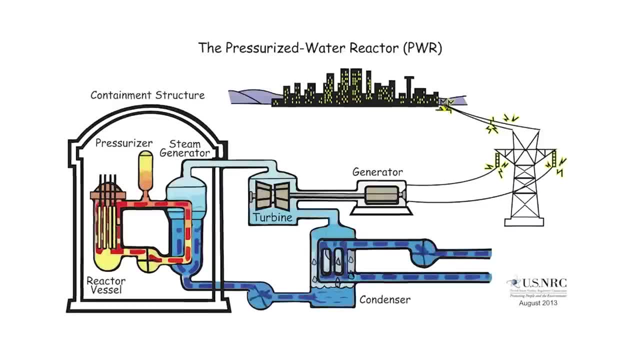 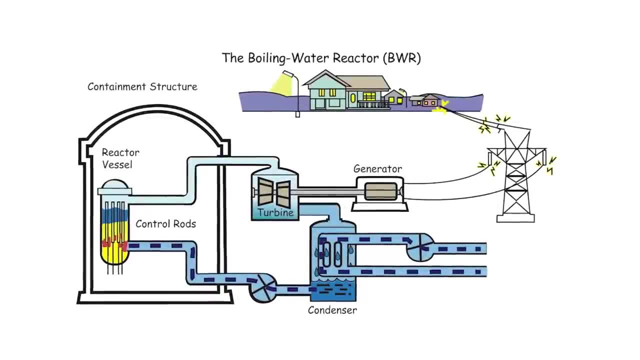 system, The secondary water system, is allowed to boil and turn a turbine. The second kind of light water reactor is the boiling water reactor, which is just what it sounds like. The primary water is allowed to boil and we use the steam from the primary water system. 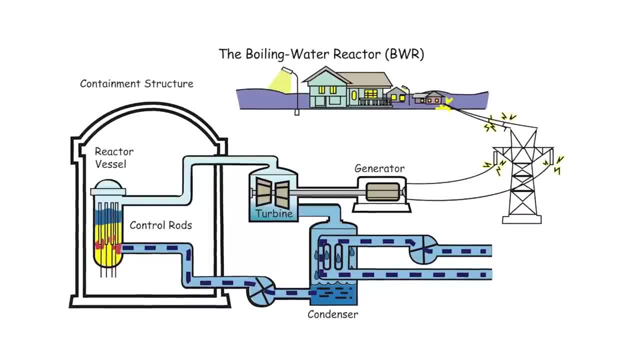 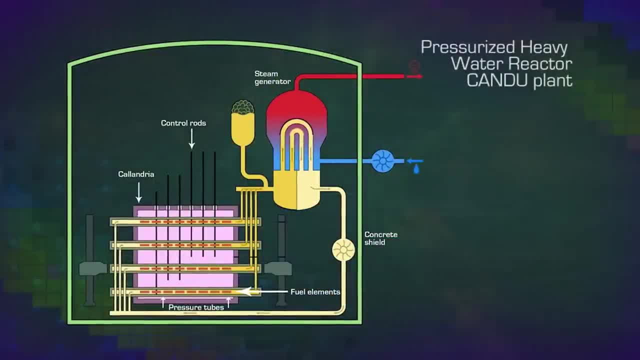 to turn the turbine and so it doesn't need a secondary water system. Then there's the pressurized heavy water reactor. It's a new plant in Canada So it uses a heavy water moderator, so that's deuterium oxide and a heavy water primary. 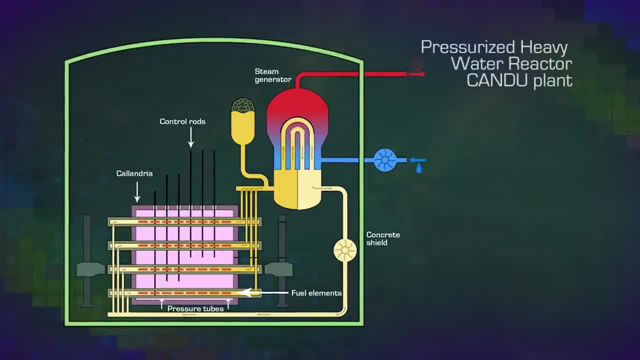 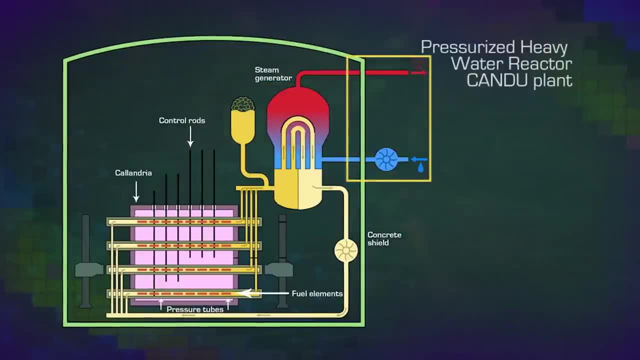 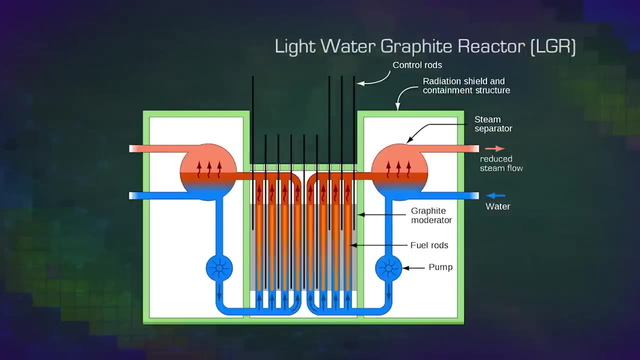 coolant, and so it can use unenriched uranium, And then the heavy water transfers its heat to a light water secondary system, which then boils and turns the turbine. There's also a water-cooled graphite-moderated reactor, And so that's similar to Fermi's original reactor- so graphite-moderated, but now it's. 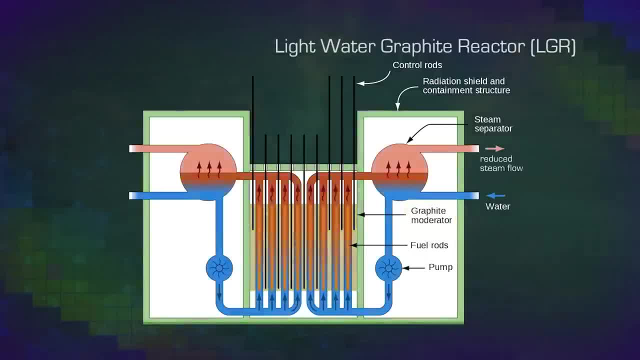 water-cooled. It can also run on natural uranium, And so that's what we're going to do: We're going to turn the turbine on. We're going to turn the turbine on. So this is the Chernobyl-type reactor, and it's built for power and for producing bomb-grade. 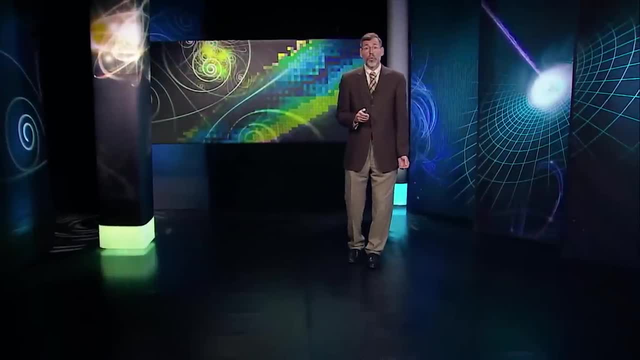 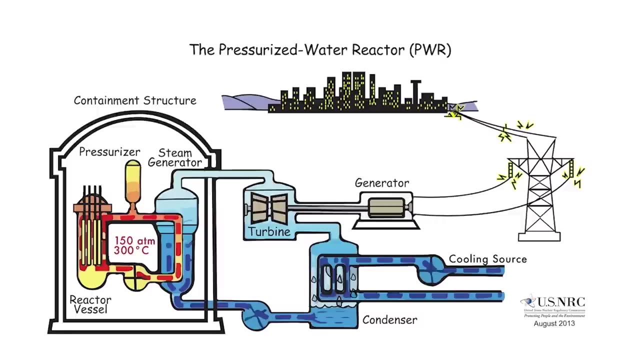 plutonium. The pressurized water reactor is the most common reactor in use today. Uses pressurized water at 150 atmospheres and about 300 degrees centigrade, which is about 600 Fahrenheit, as the coolant and the moderator in the reactor vessel. 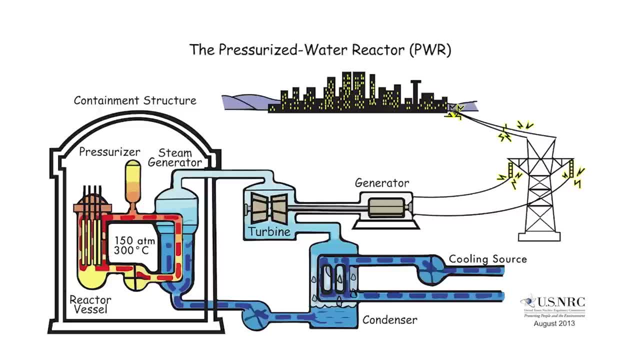 It's a closed loop. We don't let that water escape. There's a reactor pressure vessel which is about 40 feet high. It's about 15 feet high, It's about 15 feet in diameter and it's made of 8-inch-thick steel. 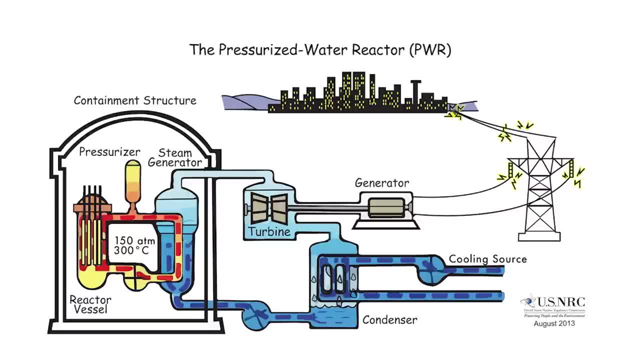 The primary water system, then transfers it to a secondary water loop in something called a steam generator, and then it has a containment building with concrete and steel to contain everything inside of it: The pressurized water reactor, then the non-nuclear part, the steam from the secondary water system. 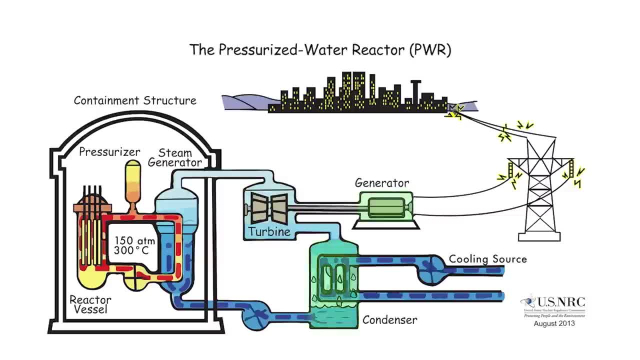 turns the turbine, The turbine turns the generator. There's a condenser that condenses the steam to make the low-pressure side of the turbine, and we need a cooling source for that condenser which, as we said, can be an ocean, a lake. 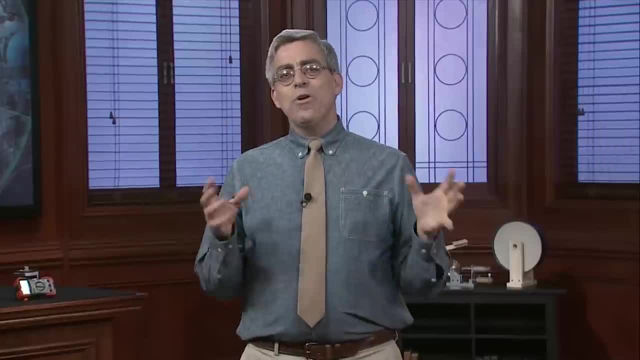 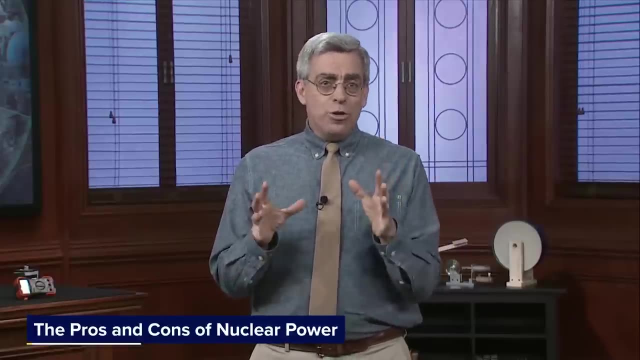 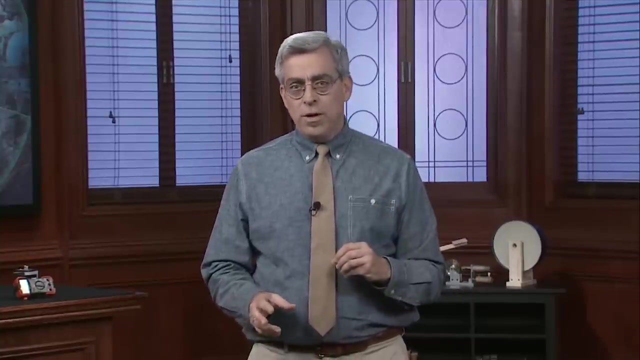 a river or a cooling tower. Now it's important to recognize that from a macro perspective, the advantages of nuclear power are considerable. Nuclear plants can operate at max capacity for extended periods of time, so they're very effective at meeting base load. 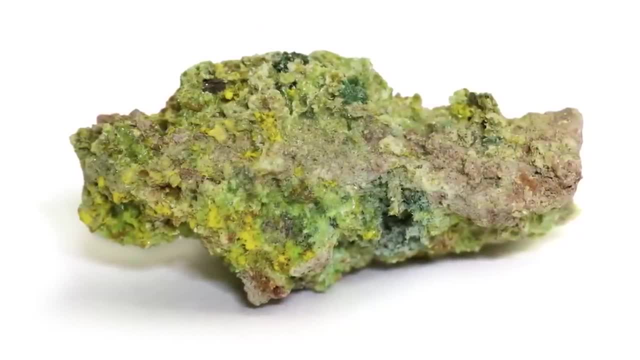 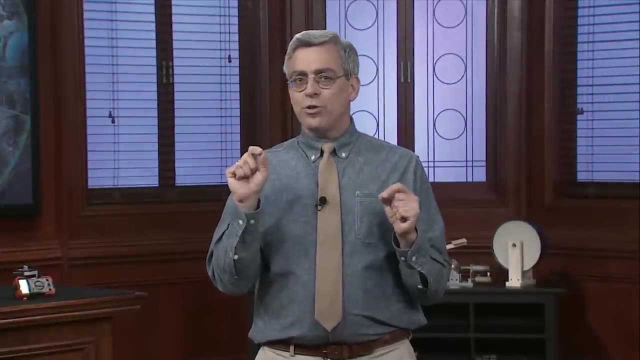 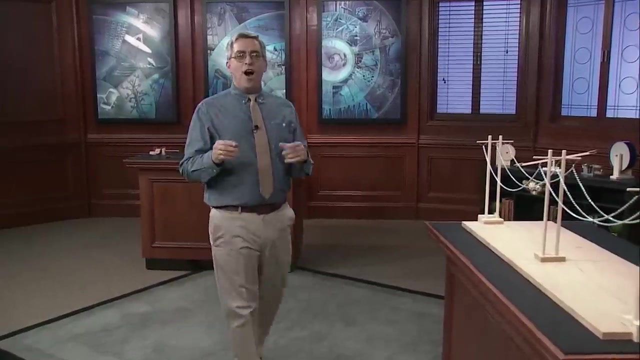 Although nuclear fuel is a non-renewable resource, there's enough of it in the Earth's crust to last for centuries. More importantly, properly contained nuclear fission produces minimal air pollution and no CO2.. In the first decade of the 21st century, a growing appreciation for these advantages. 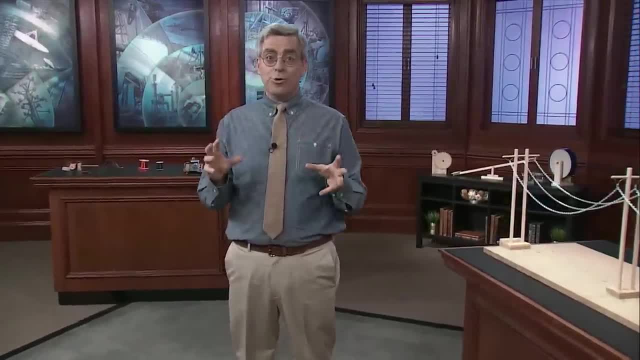 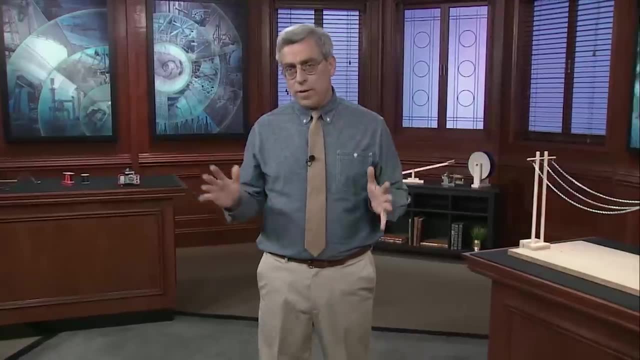 coupled with post-911 concerns about our dependence on energy sources from unstable regions of the world led to a resurgence in enthusiasm for nuclear power, both in the US and abroad. Many new power plant construction projects were initiated and there was talk of a nuclear 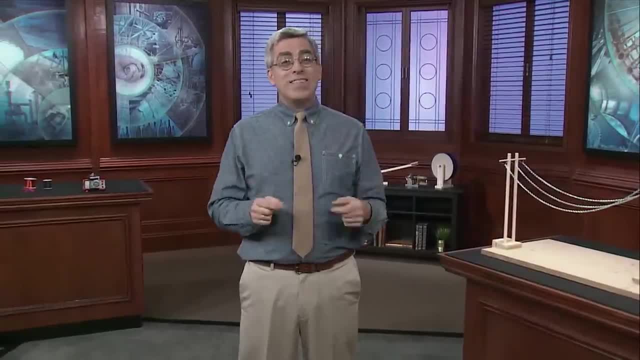 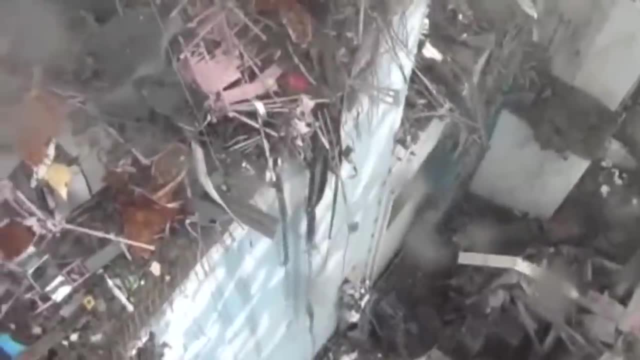 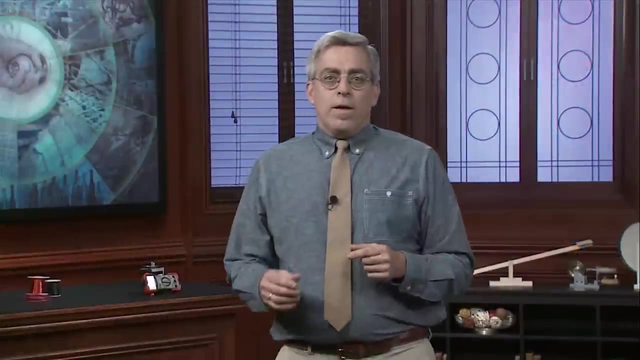 renaissance, and of nuclear power as a major component of a new, environmentally friendly power generation system. Then came the 2011 Fukushima power plant disaster, throwing the nuclear industry back on its heels once again. The Fukushima incident was triggered by a magnitude 9.0 earthquake off the coast of 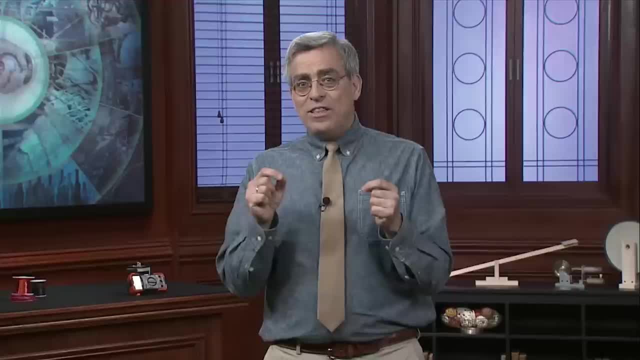 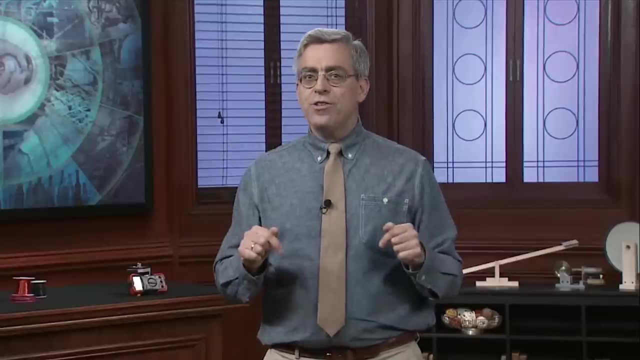 Japan. Initially, the plant's safety systems worked exactly as they were supposed to Between all three operating reactors. control rods were inserted into the reactor cores to shut down self-sustained fission, and emergency generators were switched on to power the cooling. systems. This is an essential aspect of nuclear safety because even after the control rods stop the self-sustaining fission reaction, the reactor core continues to produce tremendous heat for many hours because of continuing radioactive decay. Thus it's critical to continue coolant circulation for several days. 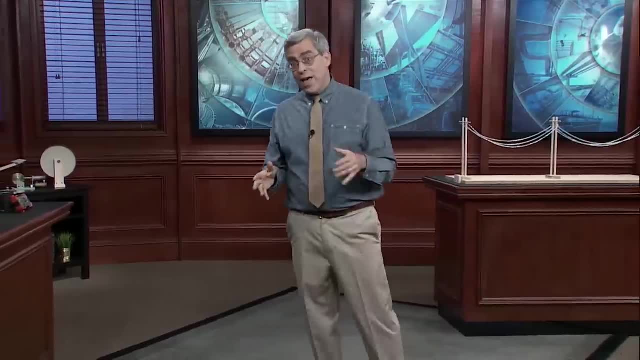 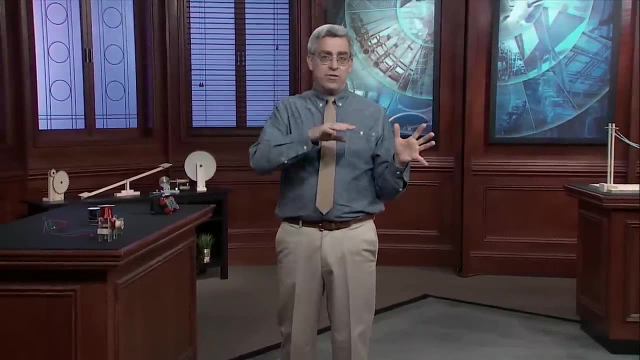 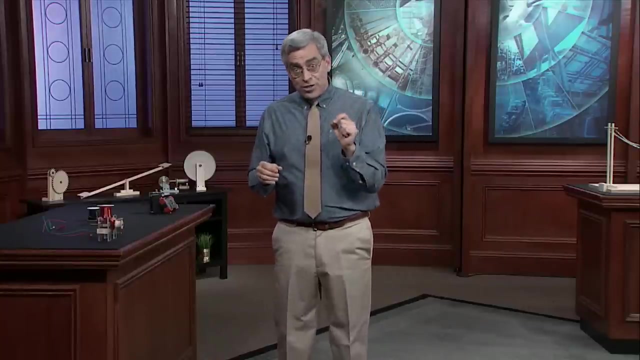 Tragically at Fukushima, 50 minutes after the earthquake, an earthquake-induced tsunami overtopped the plant's protective seawall and flooded the facility, causing the emergency generators to fail. The plant's backup battery system immediately took over, but when the batteries went dead, 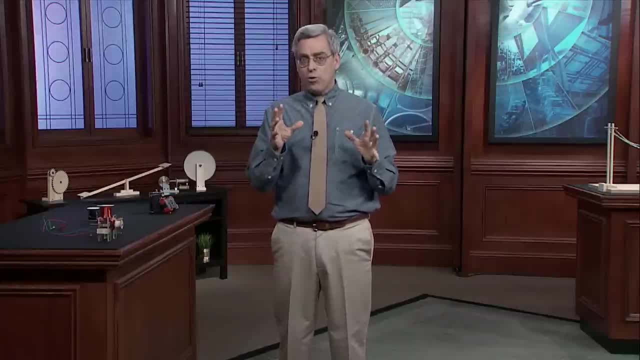 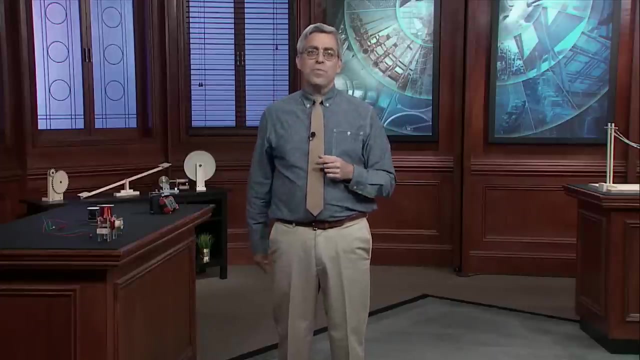 the following day, there was nothing to prevent all three reactor cores from melting down. In a meltdown, the nuclear fuel elements exceed their melting point. This caused fission products to enter the coolant water and greatly increased the possibility of a radioactive release from the containment vessel. 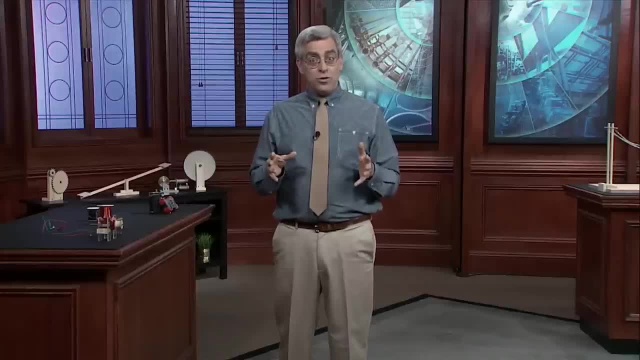 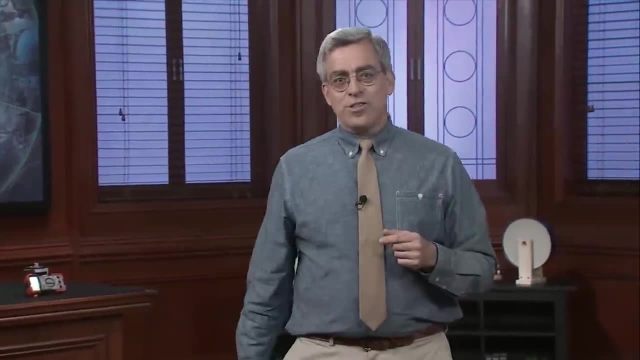 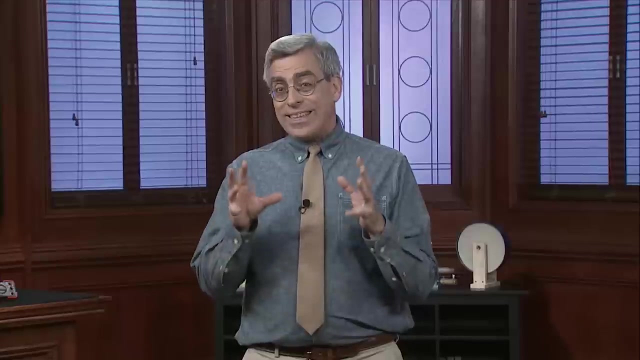 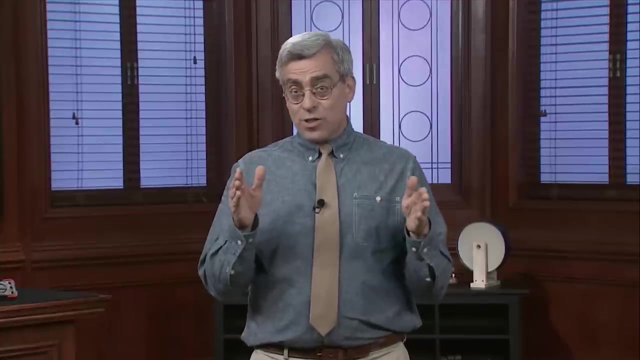 At Fukushima. the result was a humanitarian, environmental and economic catastrophe. Fukushima effectively ended the nuclear renaissance, while reminding the world that, despite stringent regulations, exacting engineering codes and extensive, redundant backup systems, nuclear accidents can still happen, And when they do, the consequences can be dire indeed. Beyond the potential for nuclear accidents, the long-term viability of nuclear power is also plagued by the still unresolved challenge of nuclear waste disposal. This challenge is exacerbated by the high level of radioactivity in the products of nuclear fission. Several of the new elements created when uranium nuclei split apart have half-lives of over. 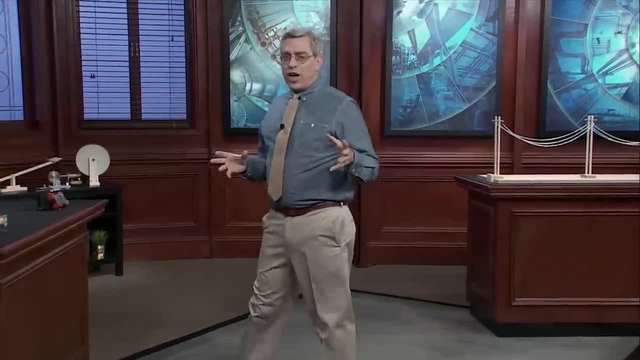 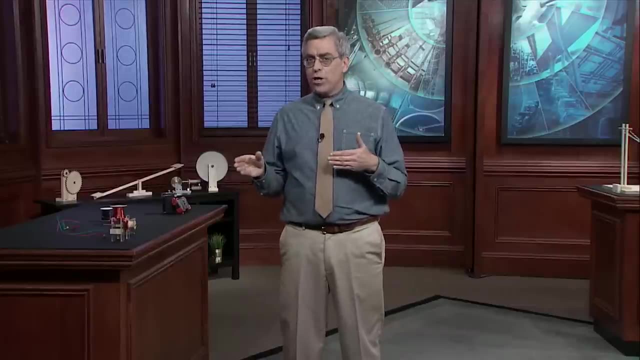 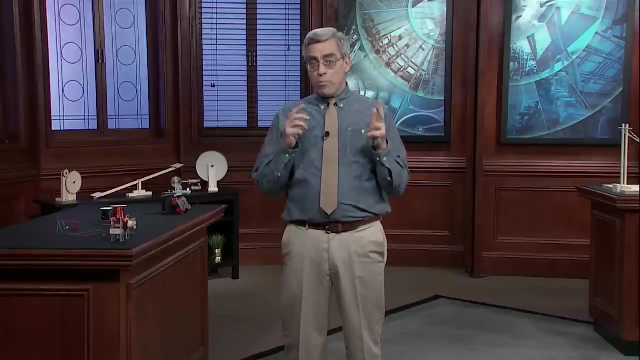 a million years. These serious challenges notwithstanding, nuclear power is not going away anytime soon. In 2012,, the US Nuclear Regulatory Commission approved the construction of four new reactors at existing power plants. China, India and South Korea are building new reactors as well. 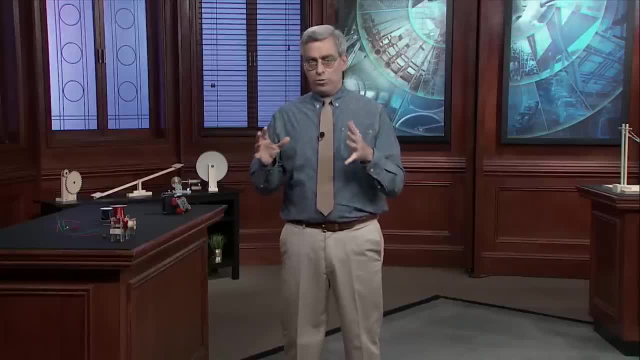 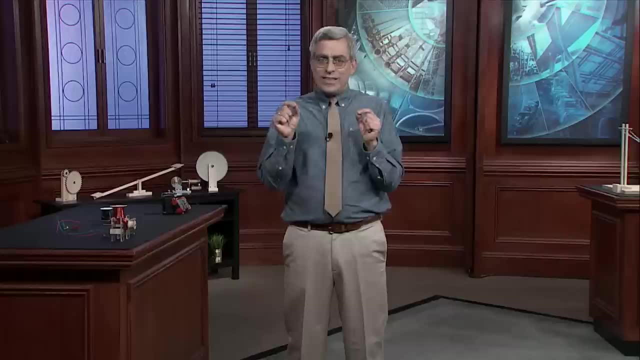 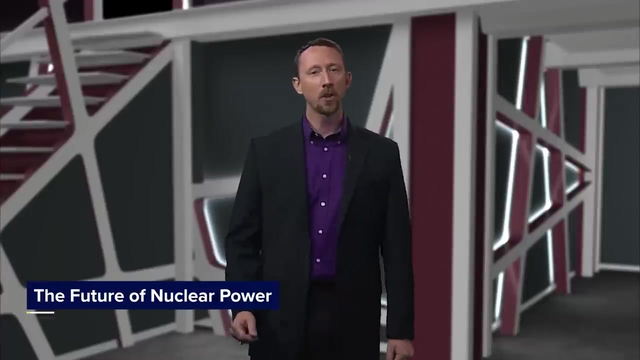 France currently generates 75% of its power with nuclear fission. And even in places where nuclear power has fallen out of favor, the immense capital investment in existing plants provides a strong incentive to keep them in operation for as long as possible. But the very obvious question remains. 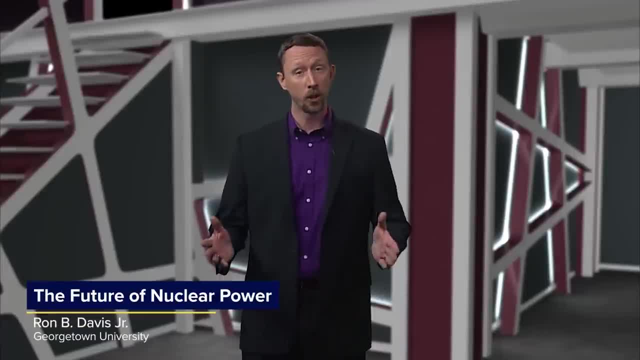 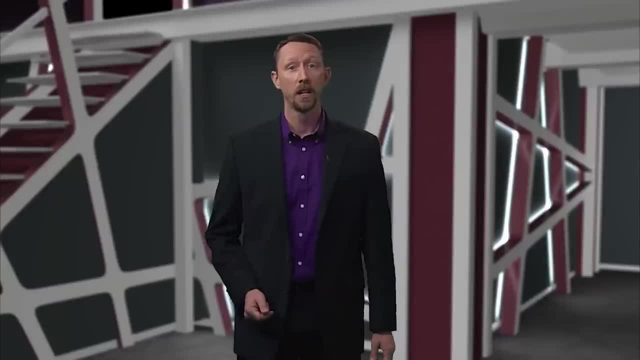 Can nuclear fusion be not only initiated but controlled? Could we somehow tap this incredibly powerful reaction the way that Fermi did with fission? It's a tantalizing prospect. Just imagine If we could tap nuclear fusion in a controlled way, not using fission bombs to initiate fusion. 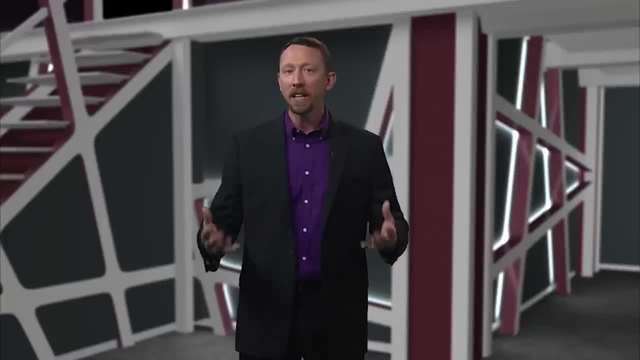 reactions that are over-the-top over in less than a second. but more elegantly conducted reaction, One in which hydrogen isotopes are fused into helium and the energy of that process is tapped. We would have power plants that use the most abundant element in the universe as fuel. and produce harmless, stable helium as waste that simply floats into space. But the problem that we run into is that even deuterium-tritium fusion, which is the easiest type of fusion reaction to start, requires temperatures about 40 million kelvins to sustain. 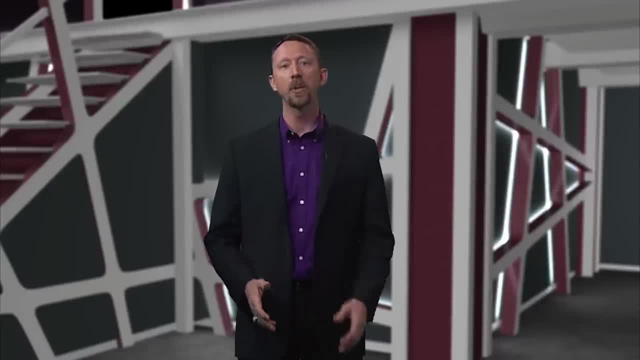 The energy needed to overcome the kalamic repulsion of the two hydrogen nuclei is just so monstrous that we can't run fusion in a power plant the way that we can do it in a bomb. There must be something fundamentally different about how a fusion reactor is designed. if 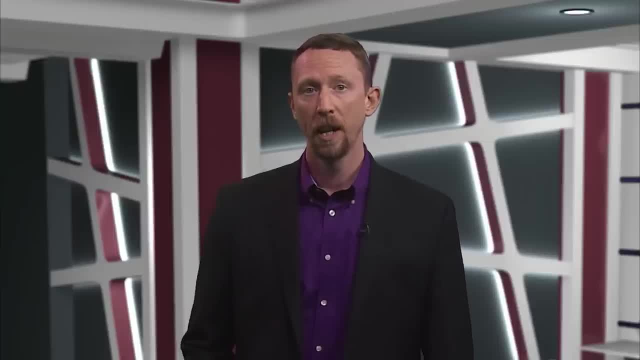 it's going to be practical for power generation. We have to find a way to run the same nuclear fusion reaction at drastically lower temperatures. We have to create a type of cold fusion. The quest for controlled nuclear fusion started about the same time that the thermonuclear. 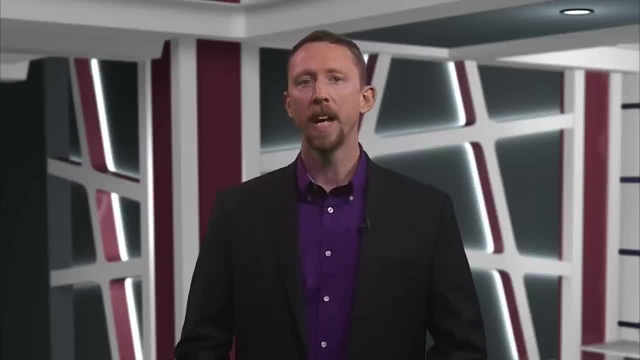 weapon or H-bomb, research began. Attempts to use magnetic fields to create containment systems capable of generating high pressures have been employed, and physicists call this the pinch technique. Although many of these types of systems have been able to contain high-energy hydrogen isotopes, they're not always the same. 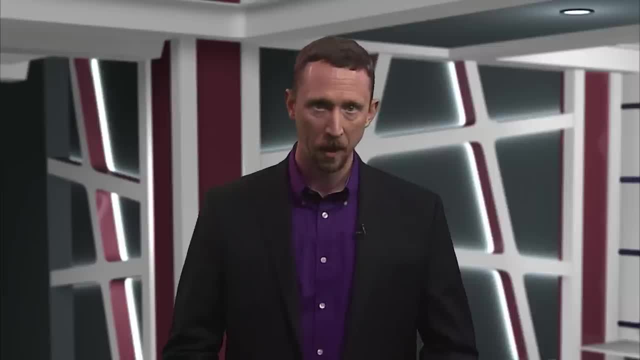 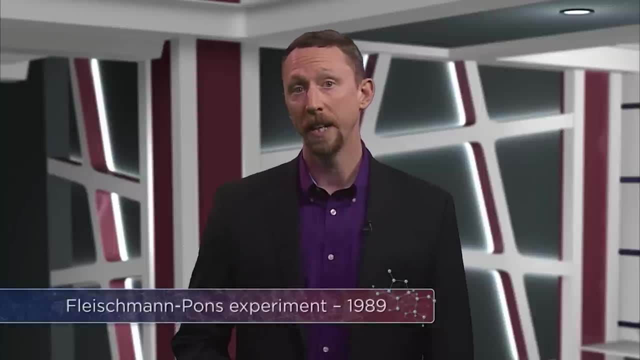 None can create the conditions right for nuclear fusion. Perhaps the most well-known story of controlled nuclear fusion is the so-called Fleischmann-Pons experiment in 1989. This experiment was a rollercoaster ride of emotion for researchers in the field, as it 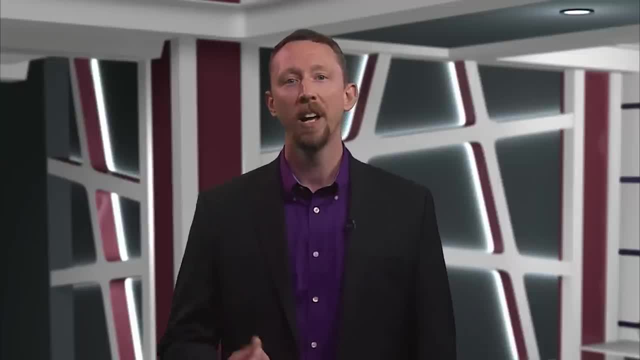 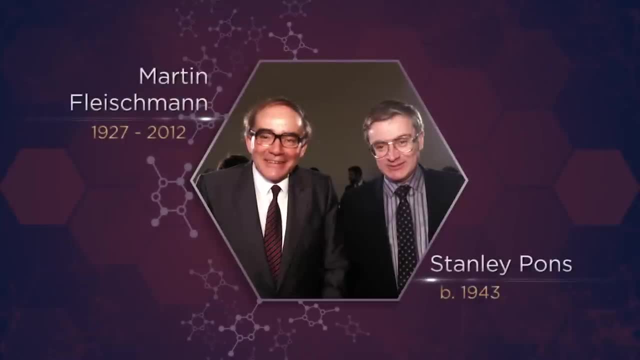 raised the world's hopes for clean, cheap fusion power, just before dashing those hopes nearly permanently. In 1989, Martin Fleischmann and Stanley Pons were conducting electrochemical experiments on nuclear fusion. They were conducting electrochemical research at the University of Utah and they believed. 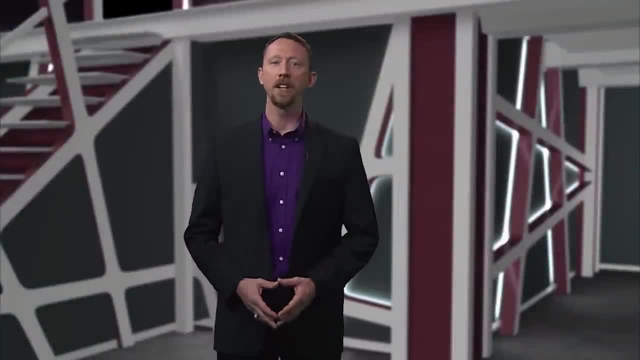 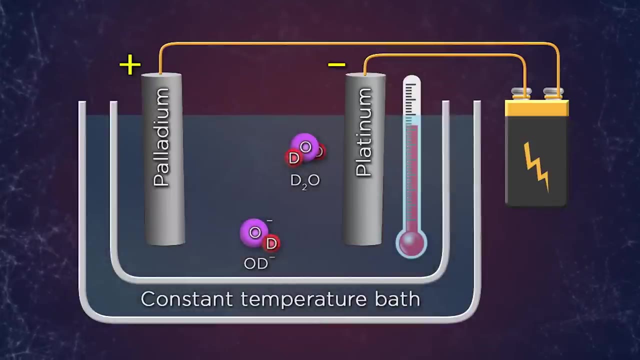 they were onto something. They had constructed a very simple device that both men believed would change the world. Fleischmann and Pons created an electrochemical half-cell using a platinum electrode submersed in what is known as heavy water or water containing deuterium instead of hydrogen. 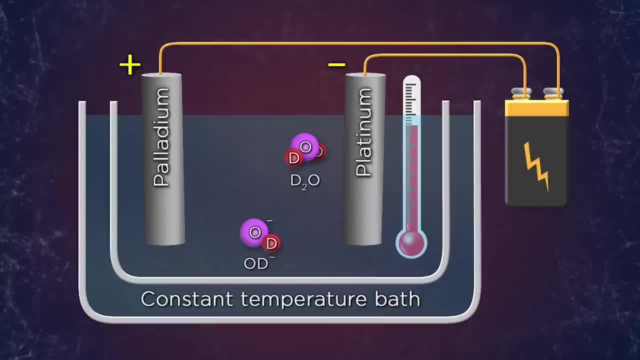 Of course the product of this half-reaction is deuterium itself, which should effervesce and bubble out of the system as deuterium. But Fleischmann and Pons had detected deuterium in the platinum electrode itself. Not a particularly surprising claim, since hydrogen gas interacts with platinum very 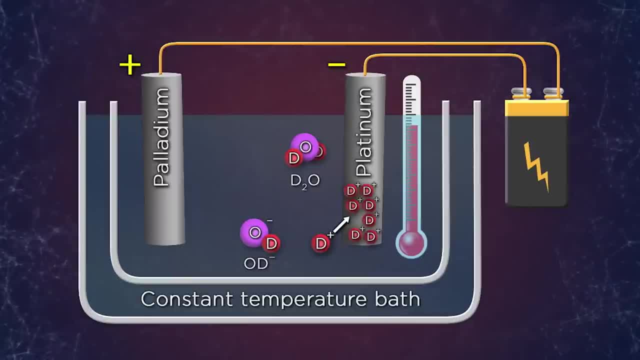 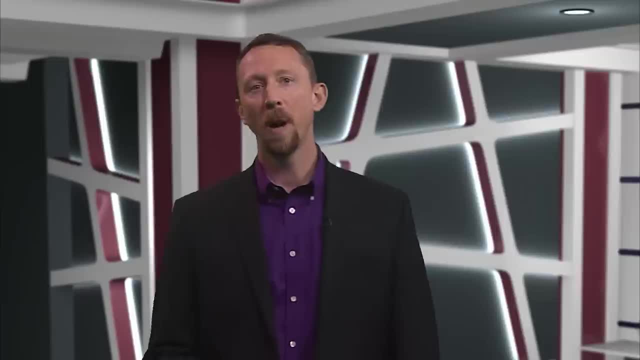 strongly adhering to its surface. But what they claimed next started a storm of scientific controversy. that's the stuff of legend. The two published a paper claiming that they had detected heat in excess of any expected chemical reaction. that would go on in their setup. 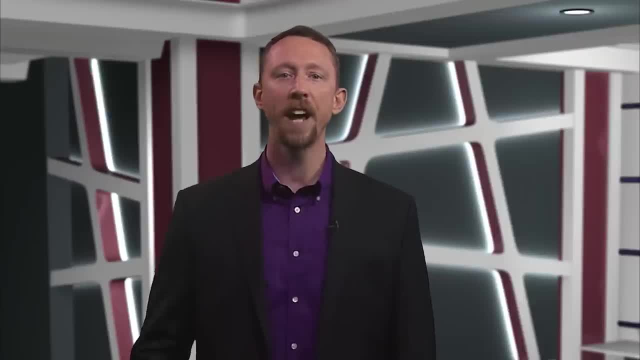 In one of the most famous papers. the paper was published by the University of Utah and it was published by the University of Utah In one of the most famous rushes to press in all of scientific history. Fleischmann and Pons let their excitement and the pressure to patent their potentially world-changing